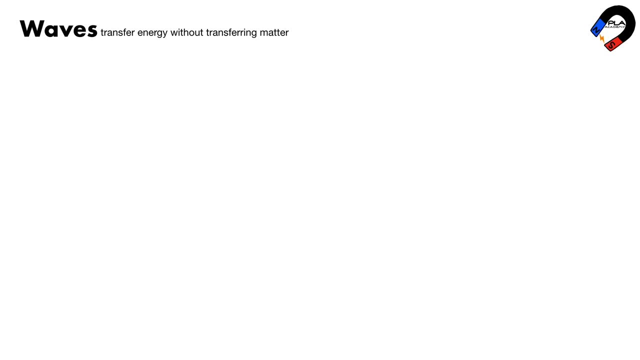 two types: transverse waves and longitudinal waves. Transverse waves: In transverse waves, the direction of vibration is perpendicular to the direction of propagation or direction of energy transfer or the direction of wave traveled, For example, water waves, seismic secondary waves, slinky waves and electromagnetic waves. We can demonstrate: 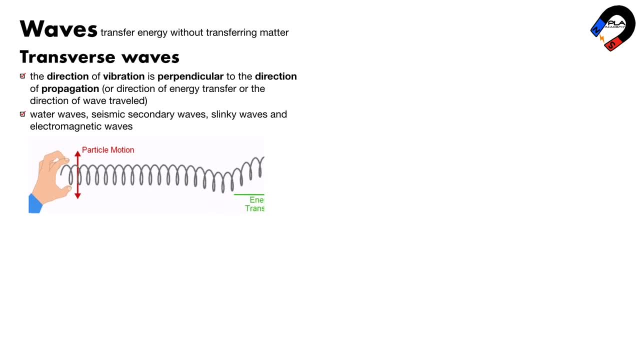 the transverse wave by shaking the spring up and down, as shown. Direction of vibration is up and down, which is perpendicular to the direction of vibration In transverse waves. the direction of wave propagation or direction of energy transfer or direction of wave traveled is to the right. 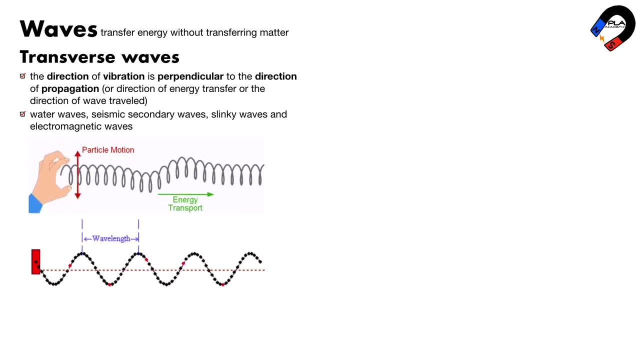 Direction of vibration is up and down around the equilibrium position. This is the equilibrium position. When the wave vibrates for one cycle, it creates one wave that travels one wavelength. The red particle at the red arrow is moving up and down. This shows that wave transfers energy without transferring matter. 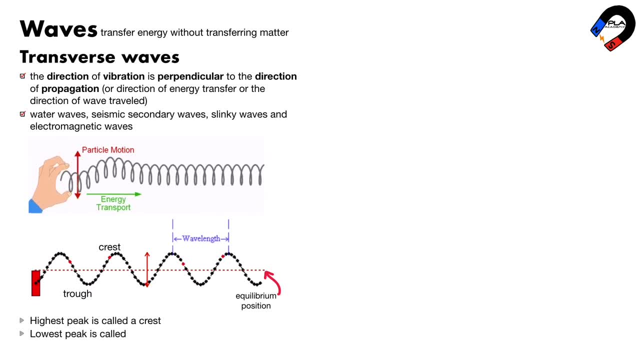 Highest peak is called a crest, Lowest peak is called a trough. Longitudinal waves: In longitudinal waves, the direction of vibration is parallel to the direction of propagation or direction of energy transfer or the direction of wave traveled, For example, sound waves, slinky waves and 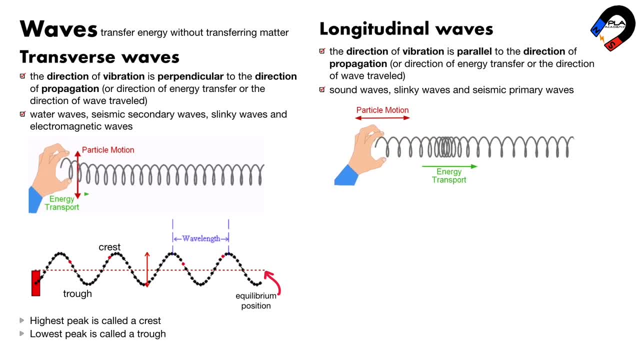 seismic primary waves. We can demonstrate a longitudinal wave by shaking the spring forward and backward as shown. Direction of vibration is forward and backward, which is perpendicular to the direction of wave propagation, or direction of energy transfer, or direction of wave traveled is to the right Direction of vibration is forward and backward around the equilibrium position. 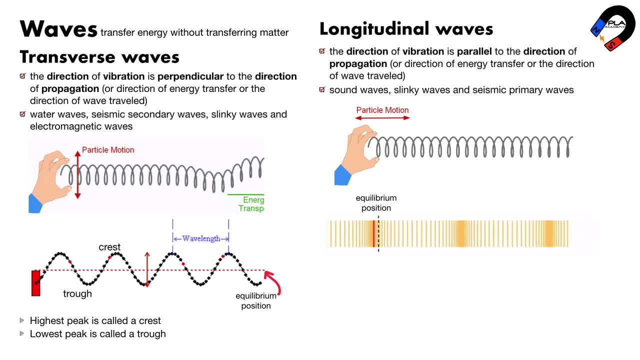 This is the equilibrium position When wave vibrate. for one cycle it creates one wave that travels one wavelength. Where the spring does not vibrate, the wave is suspended and the wave is Where the spring compresses together. this is called a compression. 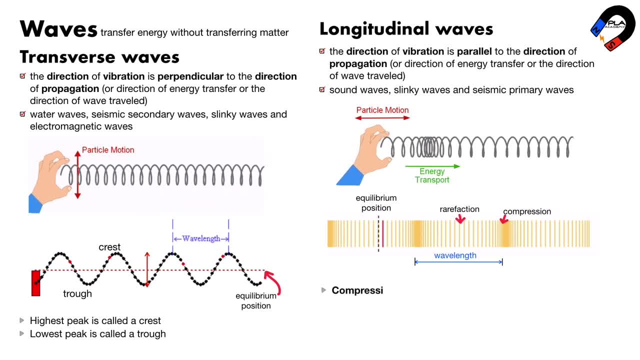 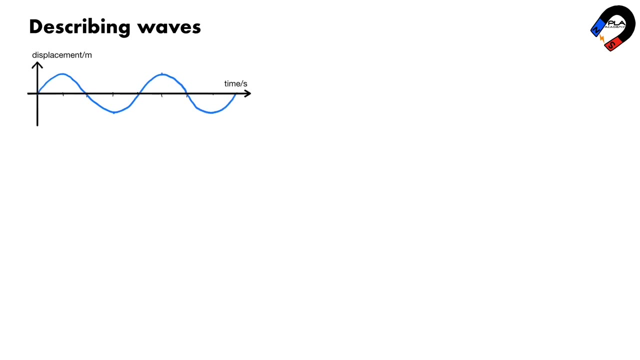 Where the spring extends apart. this is called a rarefaction. Compression is where wave particles are close together and high pressure or high density. Rarefaction is where wave particles are far apart and low pressure or low density. Describing waves: Here is the graphs of displacement: time graph of a travelling wave. 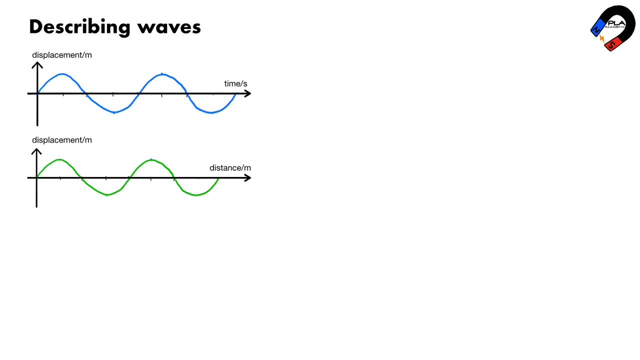 Here is the displacement distance travelled graph of a travelling wave. Amplitude A of a wave is the distance from equilibrium position to the peak of the wave. It represents energy carried by the wave, so a wave with a high amplitude carries a lot of energy. 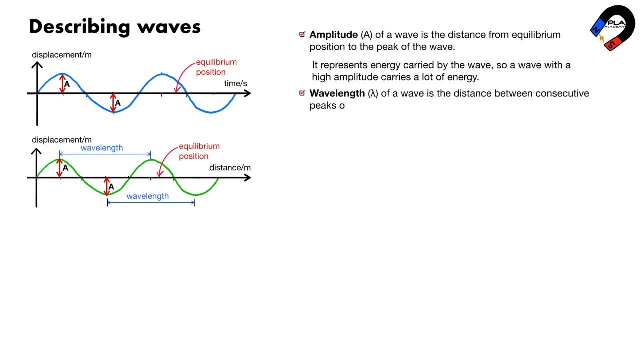 Wavelength lambda of a wave is the distance between consecutive peaks or between consecutive identical points. It is measured in metres. m. Frequency f Of a wave is the number of vibrations per second, or numbers of waves that travel past a point per second. 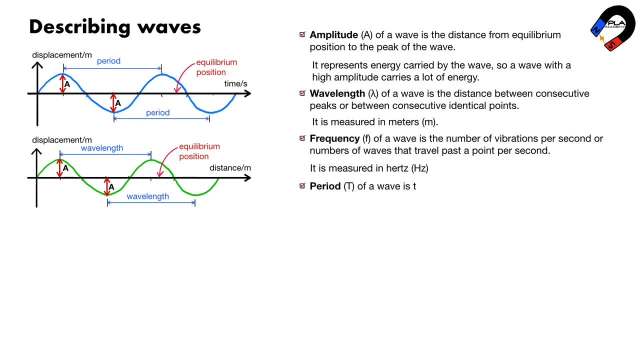 It is measured in hertz. hz. Period t of a wave is the time taken for one vibration to completely or for one wave to travel past a point. It is measured in seconds s. If a water wave travels n waves in t seconds. 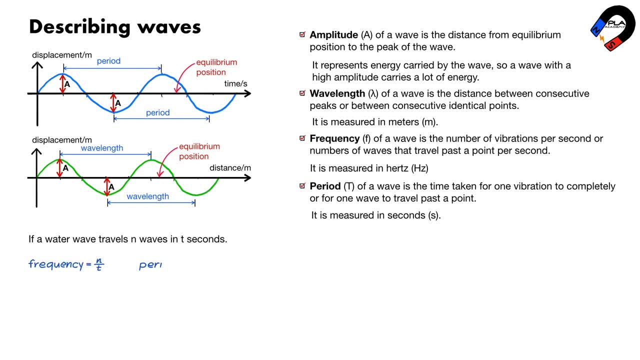 Its frequency is n to divide by t. Its frequency is n to divide by t. Its period is T to divide by N. So frequency is 1 to divide by period. Speed of a wave is the distance traveled by wavefront per unit time. 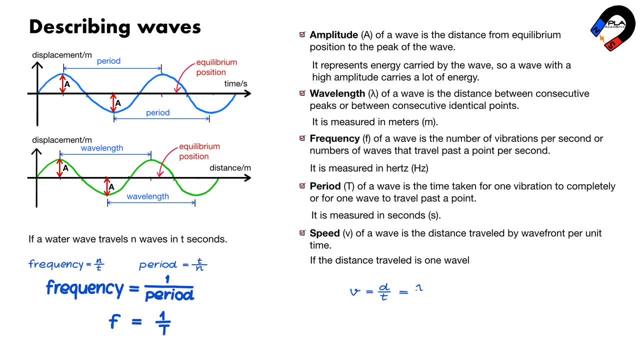 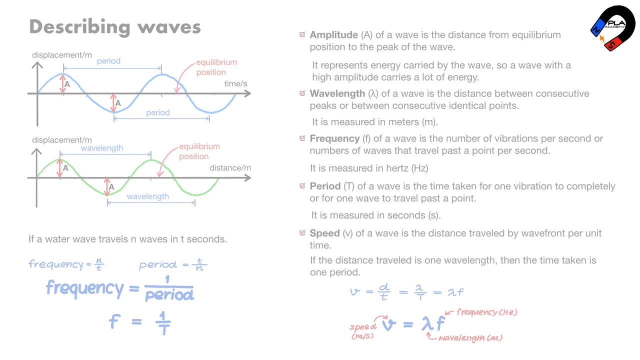 It is measured in meters per second. If the distance traveled is 1 wavelength, then the time taken is 1 period. Since 1 over period is equal to frequency, then speed is equal to wavelength times frequency. Wavefronts of wave are the lines along peaks, compressions or rarefactions of the wave. 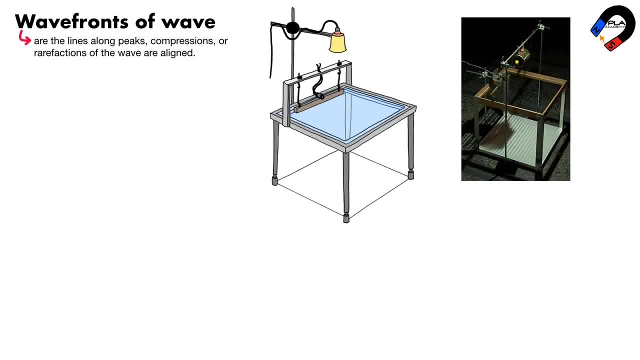 are aligned, Demonstrating the wavefronts of the water wave in a ripple tank. A ripple tank is a shallow tray of water With a light source shining down through it. The light illuminates the wavefronts, making them visible. A straight dipper can be used to create straight wavefronts in a ripple tank. 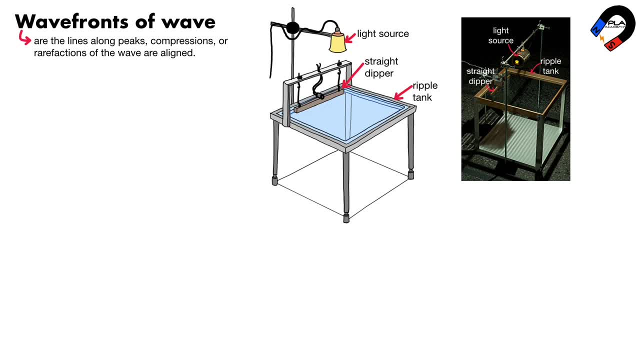 When the dipper is vibrating, the wavefronts are aligned. The dipper is vibrated up and down. It creates a series of parallel wavefronts. The screen below the ripple tank is used to observe the wavefronts of the water wave. 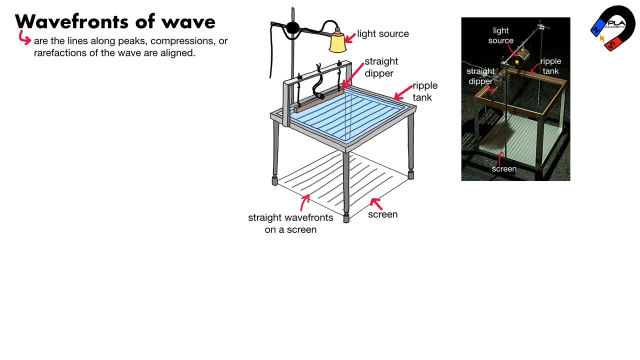 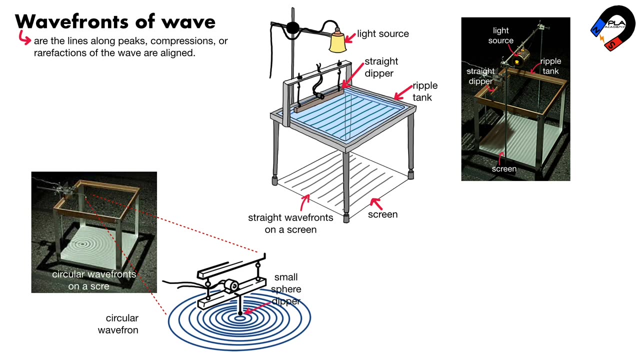 The stroboscope or video camera is used to make the slow motion of the wavefronts of water wave on the screen. A small sphere dipper can be used to create circular wavefronts in a ripple tank. When the dipper is dropped into the water, it creates a circular wavefront that expands. 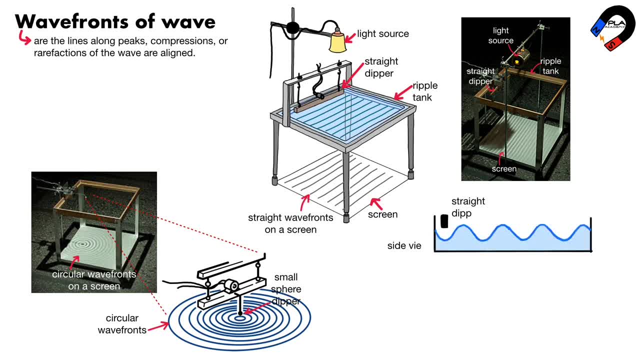 outward, As shown, The side view of the water wave in the ripple tank. The top view of the water wave in the ripple tank, We see the wavefronts are straight along crests or troughs of the wave, So the distance between consecutive wavefronts is wavelengths. 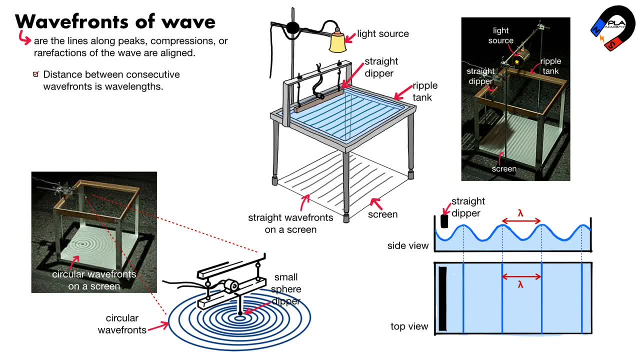 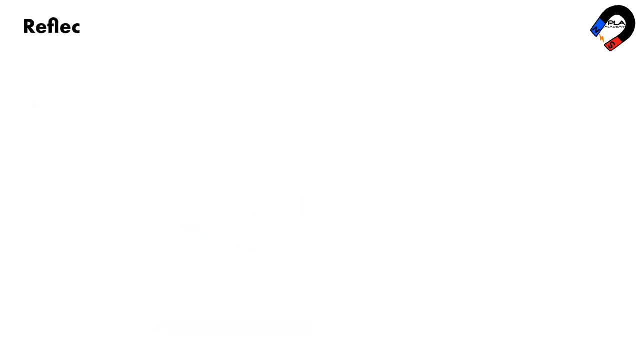 Because of the wavelength is the distance between two consecutive crests or troughs of the wave. The direction of propagation or direction of energy transfer, or direction of energy or direction of wave traveled is always perpendicular to the wave fronts. Reflection of waves: When waves hit an obstacle, they are reflected. The direction of the wave: 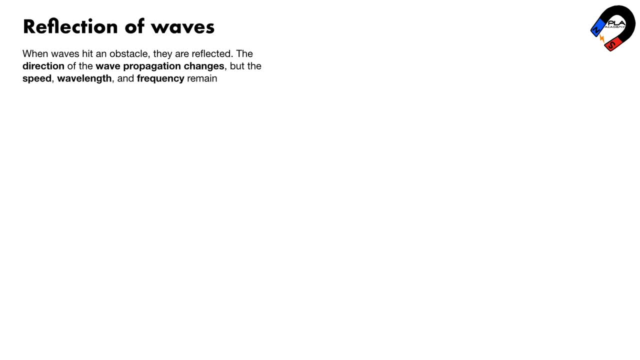 propagation changes, but the speed, wavelength and frequency remain constant. Demonstration of wave reflection using a ripple tank. The incident wave front hits the obstacle creating the reflected wave front as shown. When the series of incident wave fronts hit the obstacle creating the series of reflected wave fronts as shown, Candidates should be able to. 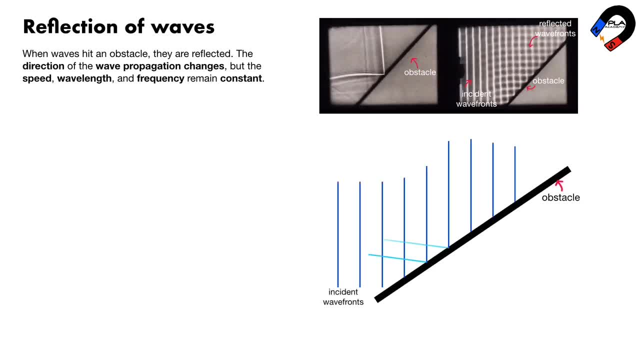 draw the diagram of this reflection. Draw the incident wave fronts and the reflected wave fronts. The angle between the incident wave fronts and the surface of obstacle is equal to the angle between the reflected wave fronts and the surface of obstacle. Draw the incident ray that is perpendicular to the incident wave fronts and its direction. 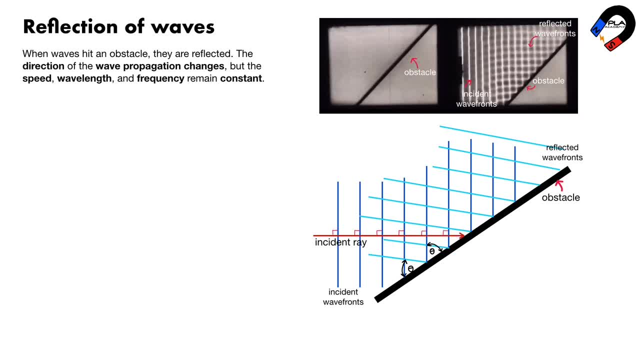 is the direction of wave propagation, direction of energy transfer. Draw the normal line at right angle to the surface of the obstacle, The angle of incidence. I is between the incident ray and normal line. Draw the reflective ray that is perpendicular to the reflected wave fronts. 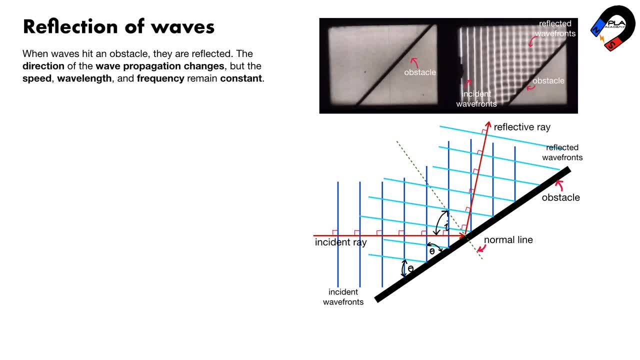 and its direction is the direction of wave propagation, direction of energy transfer. The angle of refraction R is between the reflective ray and normal line. Space between consecutive wave fronts is wavelength which are equal before and after reflection. Rules of the Reflection. The angle of incidence I is equal to: 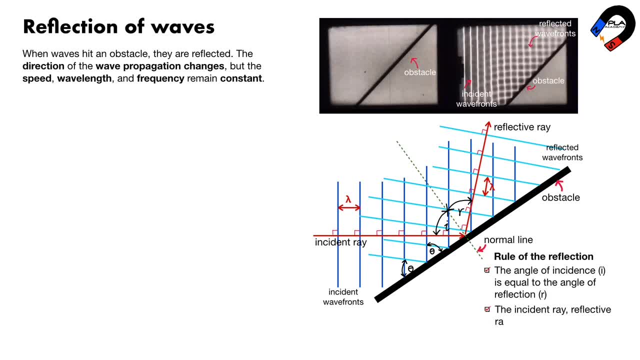 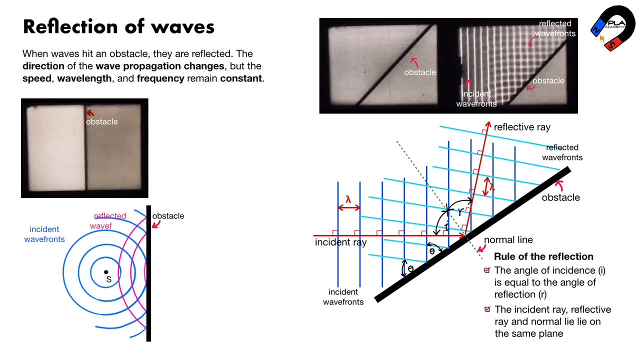 the angle of reflection R. The incident ray, reflective ray and normal lie lie on the same plane. Circular wave fronts can be reflected at a flat obstacle. as shown, The circular wave fronts is created from source. S They reflect at the flat, 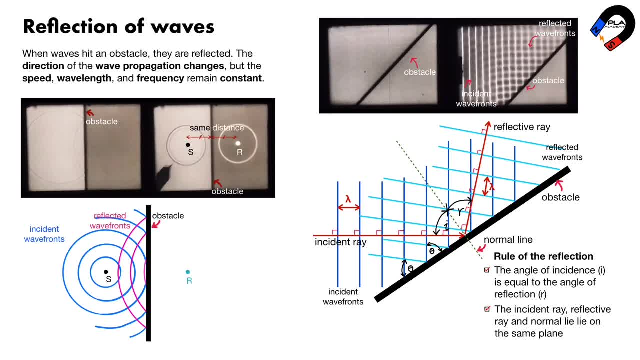 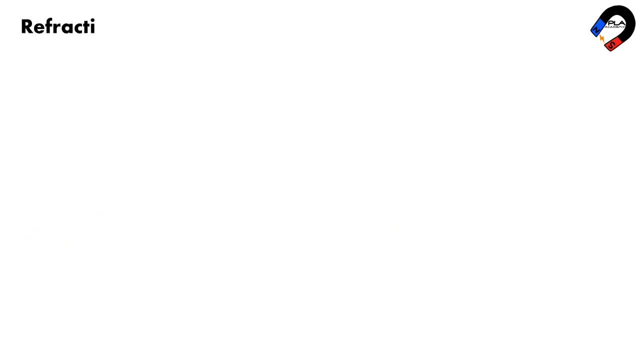 obstacle, The image of the source R is created behind the obstacle which the reflected waves appear to come. Refraction of waves: When waves travel through one medium to another, they are refracted. This is because the speed of wave is changed, causing its wavelength also change. 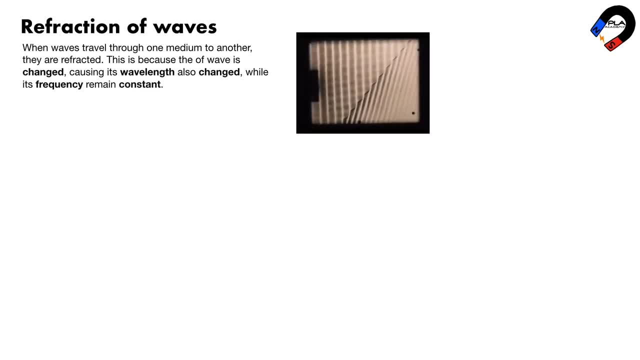 While its frequency remain constant. Demonstration of wave refraction using a ripple tank. This area is shallow water and this area is deep water. In a shallow water place the glass block in the water. The water waves travel slow in shallow water due to the friction increase. 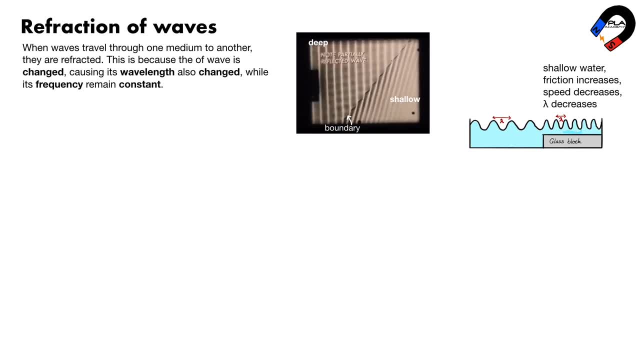 So its wavelength also decreases. while constant frequency: The water travel fast in deep water due to the friction decrease, So its wavelength also decreases. while constant frequency The incident wave fronts travel from deep water to shallow water. The wave speed decreases to cause the wave front spend towards the normal line and they are close together. This causes the 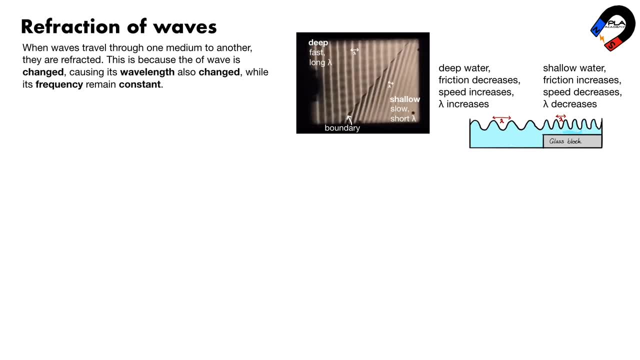 wavelength to decrease. Candidates should able to draw the diagram of the refraction of waves. This is the boundary between shallow and deep water. This region is deep water. This system is. This region is shallow water. Draw the incident wave fronts of wave in deep water. 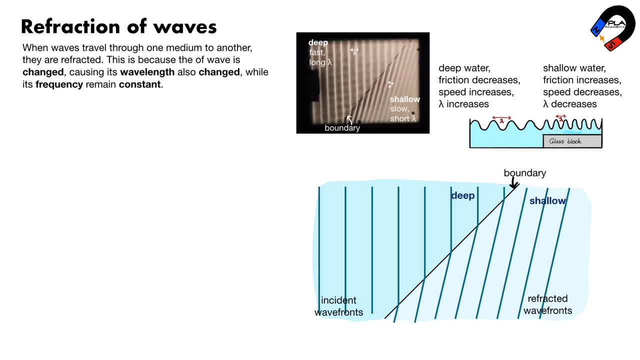 Draw the refractive wave fronts of wave in shallow water. Draw the direction of incident ray at perpendicular to the incident wave fronts. Draw the normal line at perpendicular to the surface of the boundary. Draw the refractive ray at perpendicular to the refracted wave fronts. 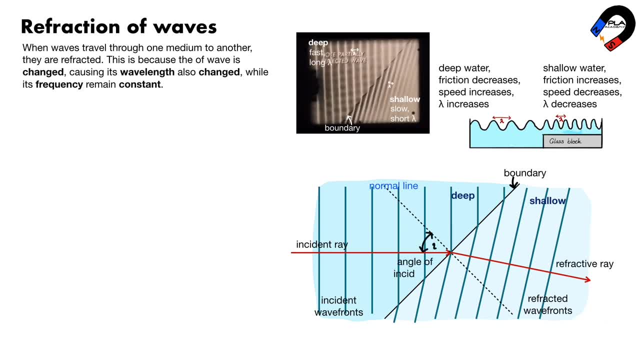 The angle of incidence I is between the incident ray and normal line. The angle of refraction R is between the refractive ray and normal line. When the water wave travel from deep water to shallow water at perpendicular to the surface of boundary, as shown, This region is: 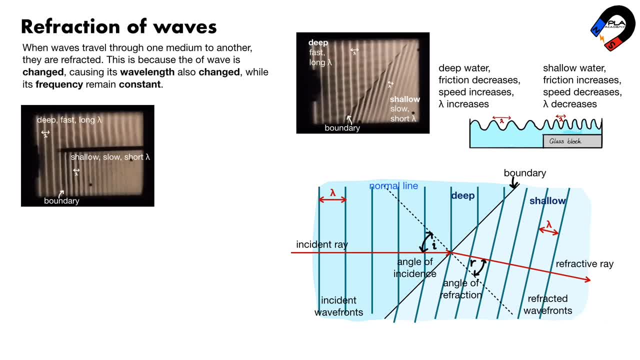 shallow water. This region is deep water. The wave fronts are not bend, but the wave fronts are close together. This shows that wavelength decreases due to the wave speed decreases when travel from deep to shallow water. Draw the diagram to show the refraction of wave of this situation: This region. 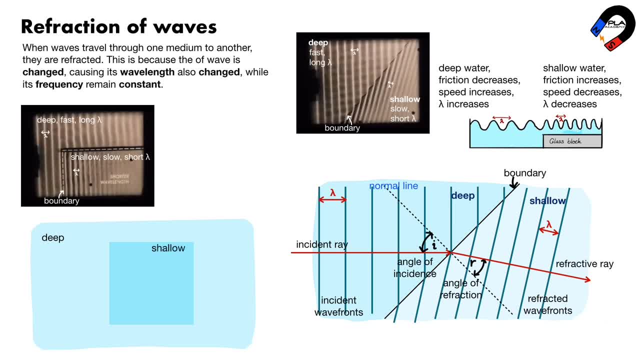 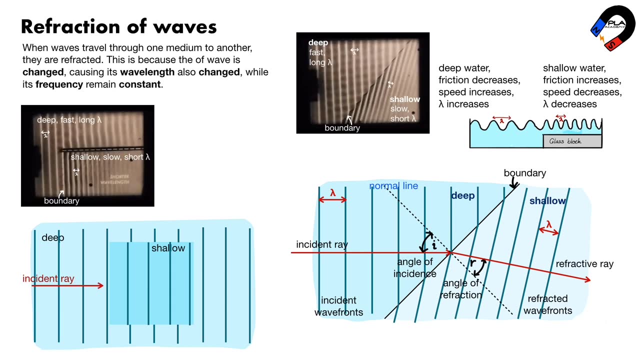 is deep water. This is region is shallow water. Draw the incident wave fronts of wave in deep water. Draw the refractive wave fronts of wave in shallow water. Draw the direction of incident ray at perpendicular to the incident ray. at perpendicular to the incident ray. 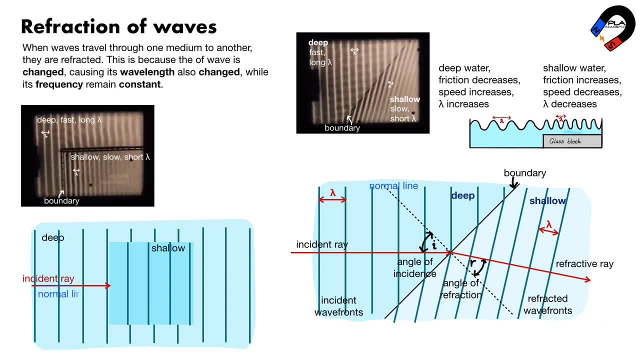 The angle of incidence I is between the incident ray and normal line to be zero. The angle of refraction I is between the refractive ray and normal line to be zero. Therefore, the refractive ray is not bend when the incident ray travels along the normal or perpendicular surface of the boundary. 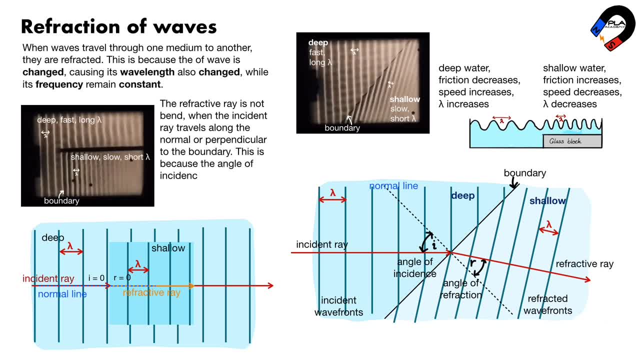 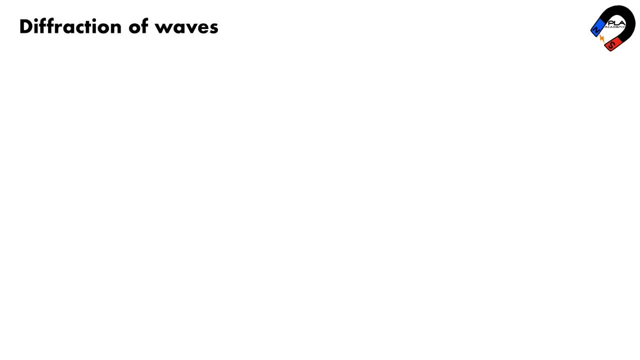 This pointsедume makes the angle of regular flow of the reflection radicular to the boundary. This is because the angle of incidence and angle of refractive are equal to zero. Diffraction of the waves is to lose any data. The speed, wavelength and frequency of the waves are constant as p. 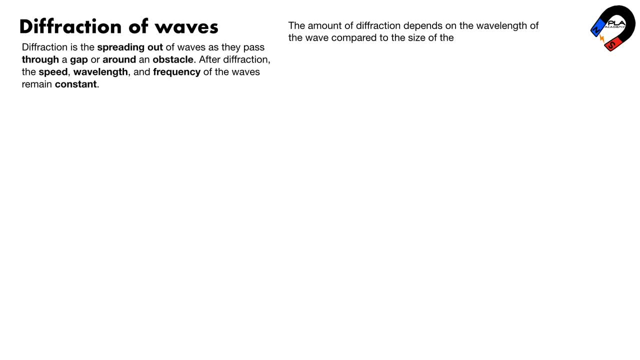 fa, f, wi, f, is2dc. Diffraction is the spreading out of waves as they pass through a gap or obstacle. More diffraction occurs when the wavelength is similar to the size of the gap or obstacle. Less diffraction occurs when the wavelength is much smaller than the size of the. 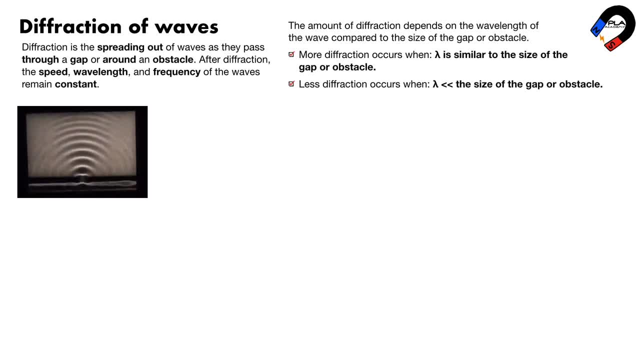 gap or obstacle. Demonstration of wave diffraction using a ripple tank. When the size of gap is similar to wavelength, as shown, Straight wave fronts pass through the gap. Waves spread out more, causing the straight wave fronts to become curve. Space between each wave fronts are equal. 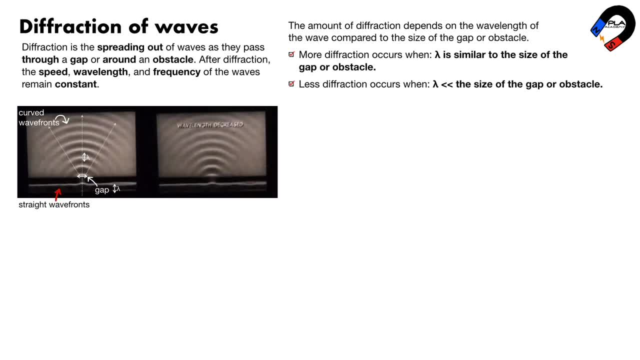 This shows that wavelength remains constant When the wavelength decreases, while the size of gap remain constant. as shown, Waves spread out less, causing the refractive wave fronts are less curved. This shows that the waves diffracted less. Candidates should be able to draw the diffraction.